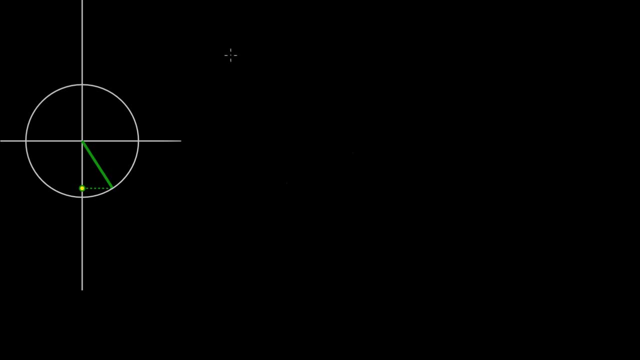 Now I'd like to demonstrate one way to construct a sine wave. What we're gonna do is we're gonna construct something that looks like sine of omega t. So we have our function of time here And we have our frequency. Now this little animation is gonna show us a way. 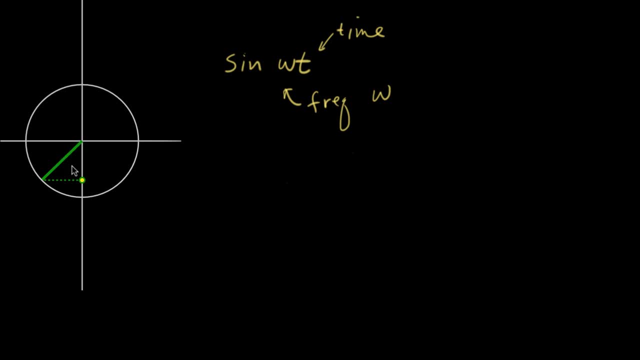 to construct a sine wave. So what I have here, this green line, is a rotating vector, And let's just say that the radius of this circle is one. So here's a vector just rotating slowly, around and around, And in the dotted line here. 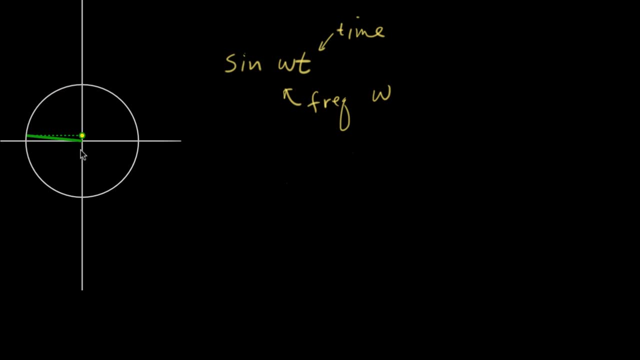 in that yellow dot going up and down. that's the projection. that's the projection of the tip of the green arrow onto the y-axis And as the vector goes round and around, you can see that the projection on the y-axis is bobbing up and down. 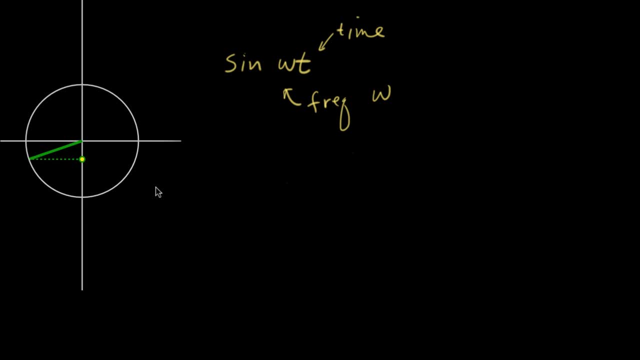 And that's actually going up and down in a sine wave pattern. So now I'm gonna switch to a new animation and we'll see what that dot looks like as it goes up and down in time. So here's the plot. Here's what a sine wave looks like. 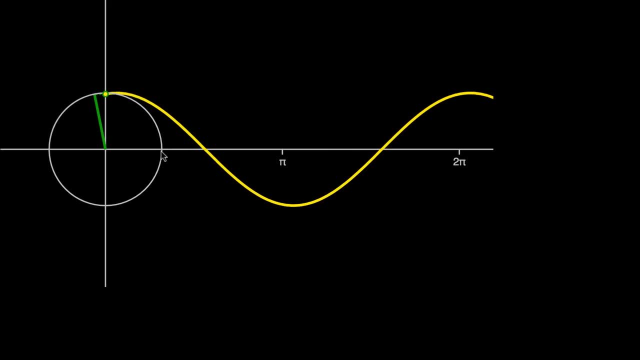 As you notice, when the green line goes through zero- right there, let's wait until it comes around again- the value of the yellow line when it goes through zero is zero. So this yellow line here is a plot of sine, of omega t. 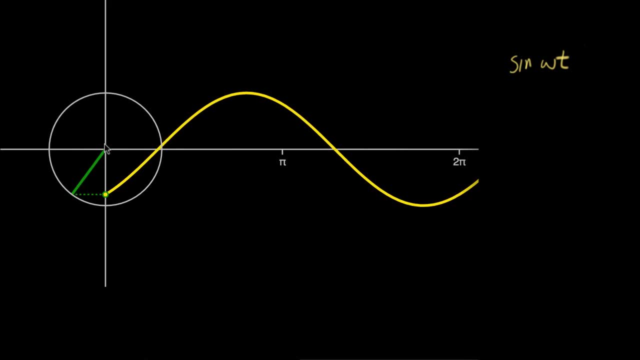 Now, if I go to a projection- this projection was onto the y-axis And I can do the same animation, but this time project onto the x-axis And that'll produce for us a cosine wave. Let's see what that looks like. 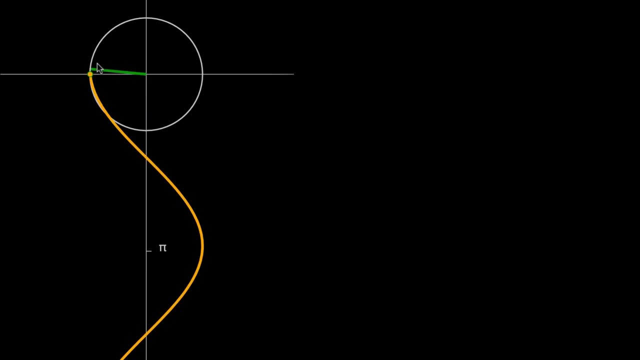 Now, in this case, if we switched over, you can see that the projection that dotted green line is onto the x-axis, And what this is doing is it's producing a cosine wave for us. So this is gonna be cosine of omega t. 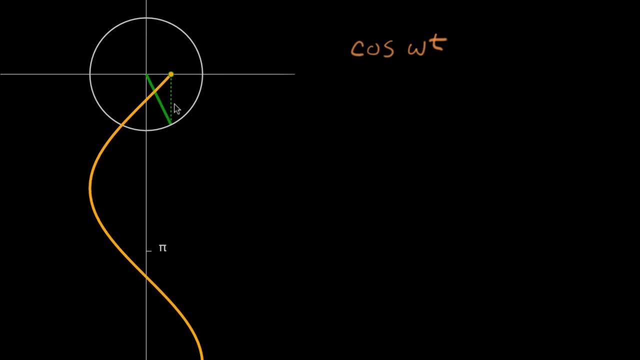 Now, because we're tracking the progress on the x-axis, the cosine wave seems to emerge going down on the page. So the time axis is down here And then we're gonna go down When the green arrow is zero. right there the value of the cosine was one.